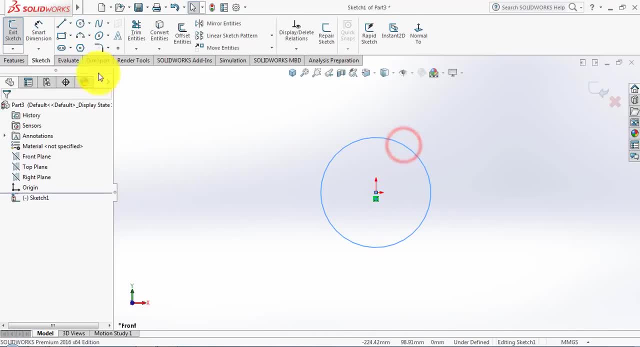 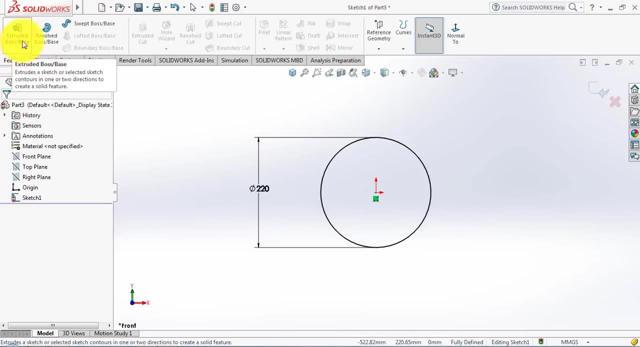 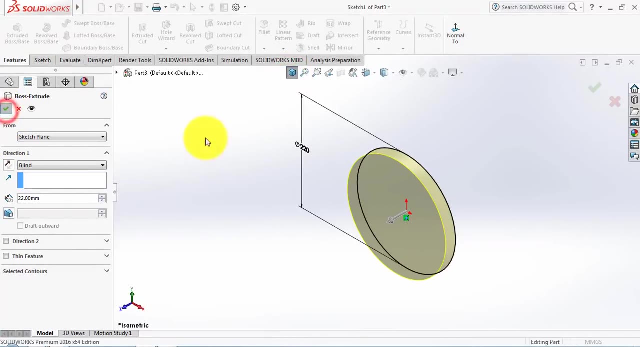 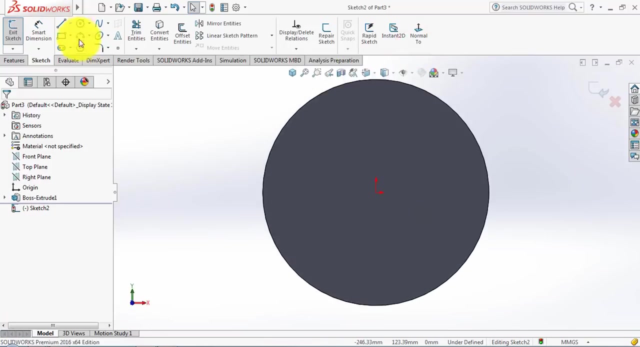 draw a circle of diameter 220 mm. Now we will go to the features and select texture, head pose feature and give the depth as 22 mm. Ok, Now again go to the sketch and select this face, Make it normal. Now here, draw a circle. 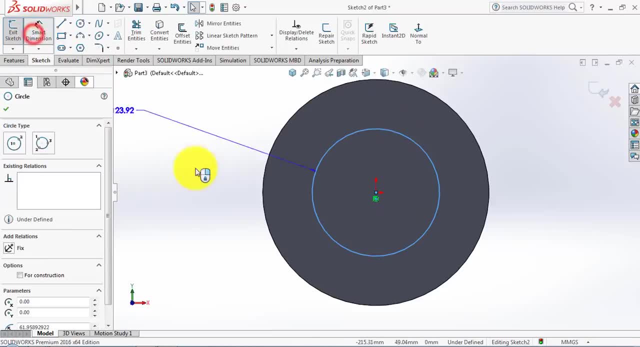 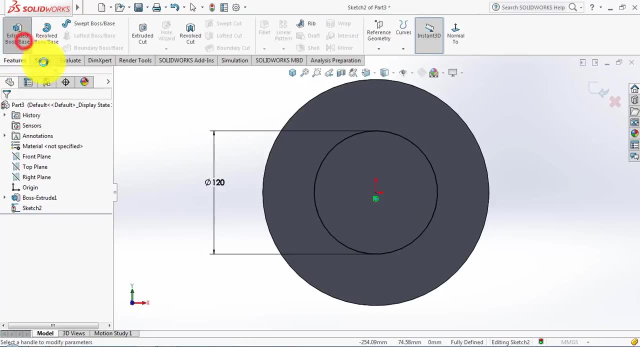 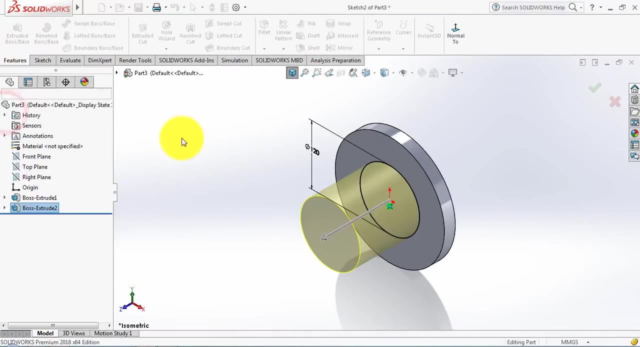 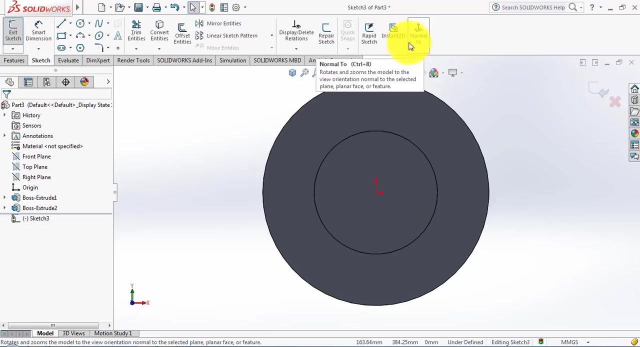 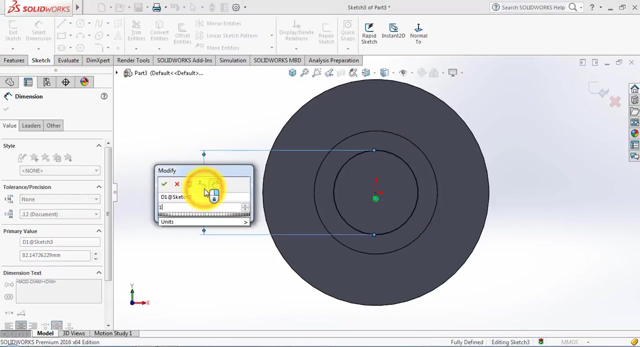 of diameter 120 mm. Now we will go to the features and select here the texture head pose feature and give the depth as 120 mm. Ok, Now again go to the sketch and select this face, Make it normal, And here we will draw a circle of diameter 100 mm. And now we will go to. 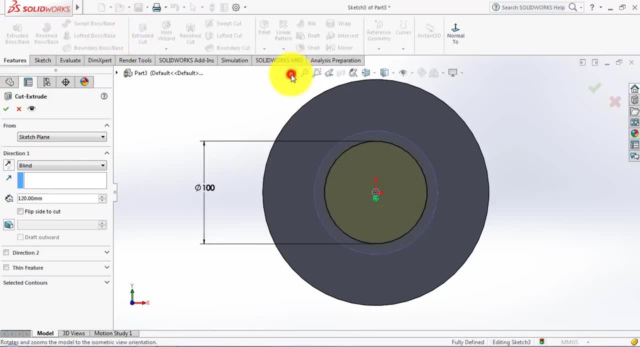 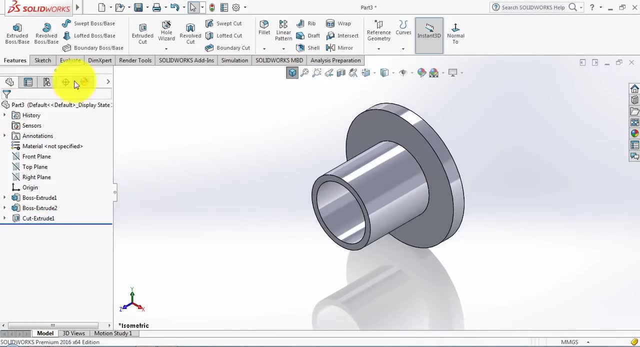 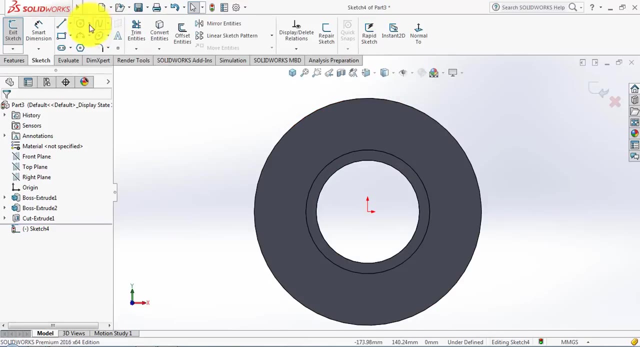 the features and select here the texture head pose feature and select here the wall. Ok, Now we will go to the sketch and select this face, Make it normal. Now, here we will draw a circle of diameter 120 mm and this will create a bright yellow color on our 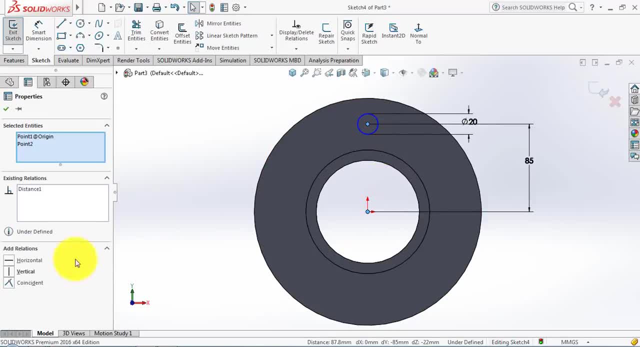 canvas. Now we will give the thickness here 0.5 inches. Ok, Now draw a circle ahead, i mean from the center. Ok, Now hold shape. I mean pull the circle towards the center and make it horizontal. We will slightly move this circle from the center and put in the 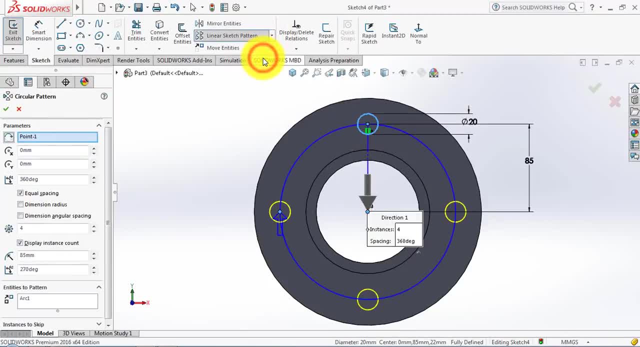 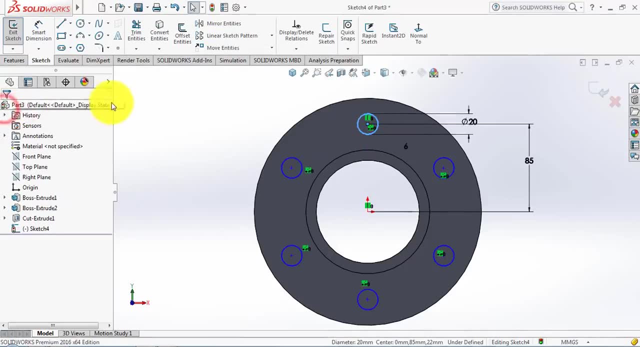 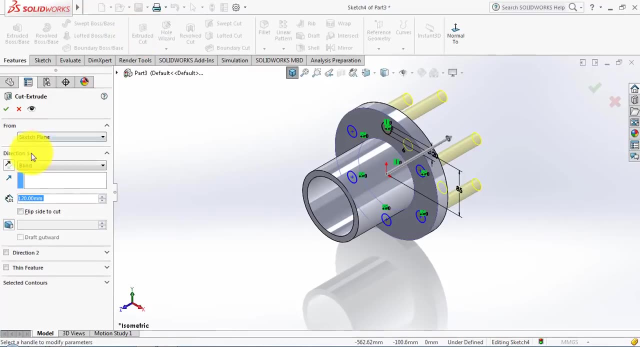 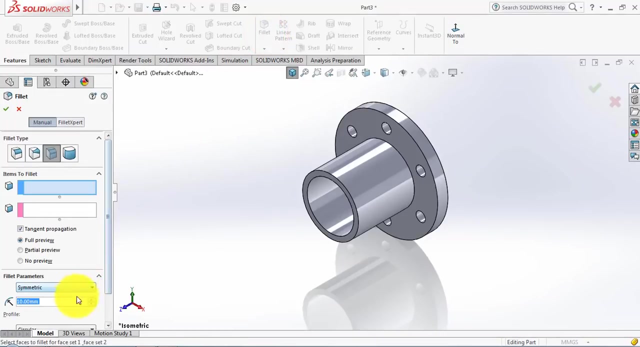 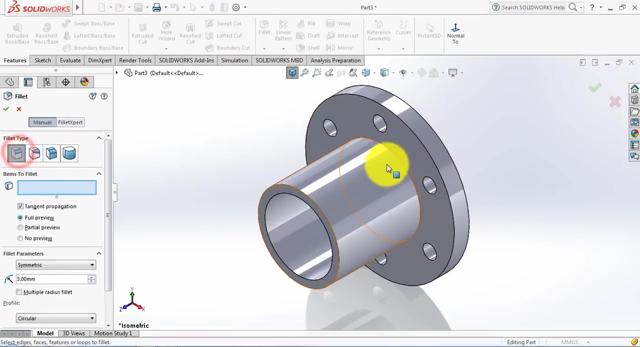 go to the circular sketch pattern and give here 6 such circles, ok. and now we will go to the features and select here the X-ray cut feature and select here through all, ok. and now we will go to fillet and give the fillet radius as 3mm and select here this: 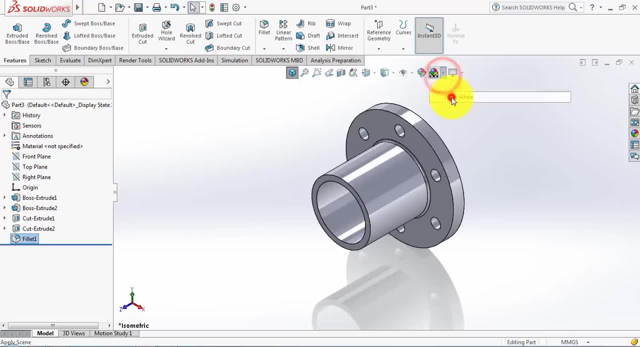 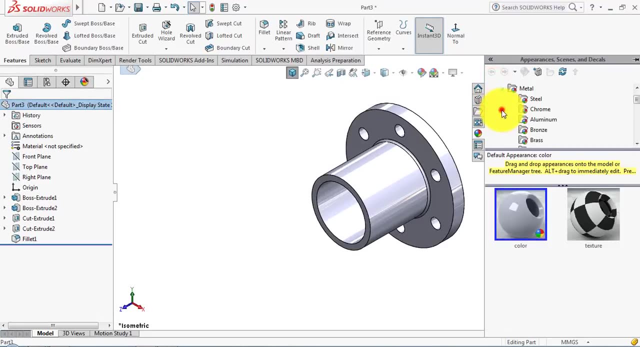 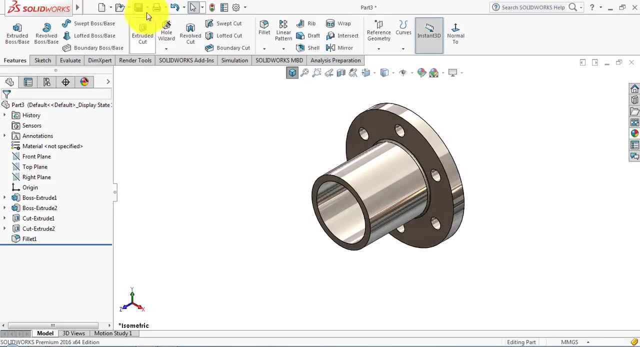 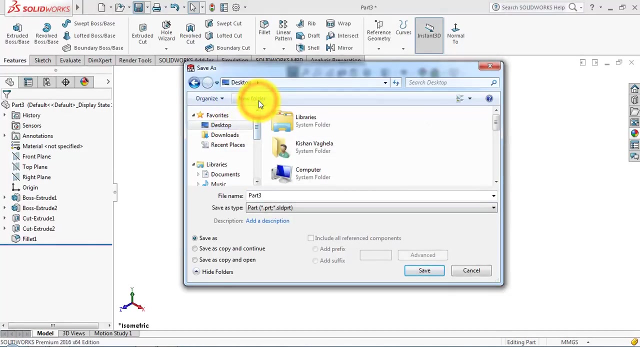 edge, this edge. ok, now we will make here the plain white. then select here the part, go to the appearance, select here the metal steel and give it here the polysteel, and now we save it. go to the service. now select here the desktop and on the desktop we will create a new folder. 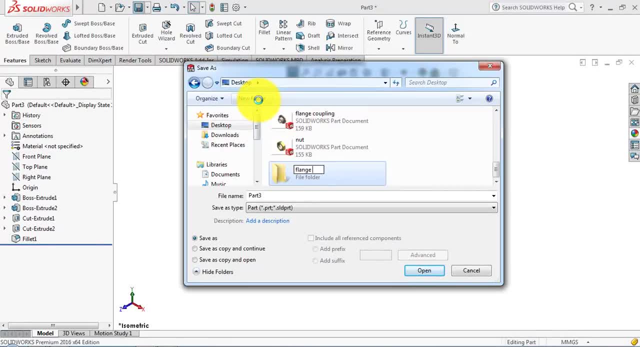 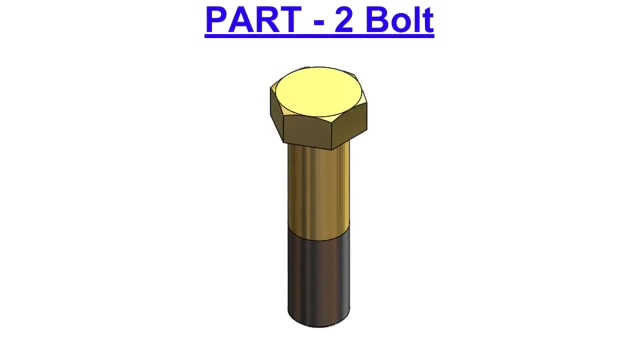 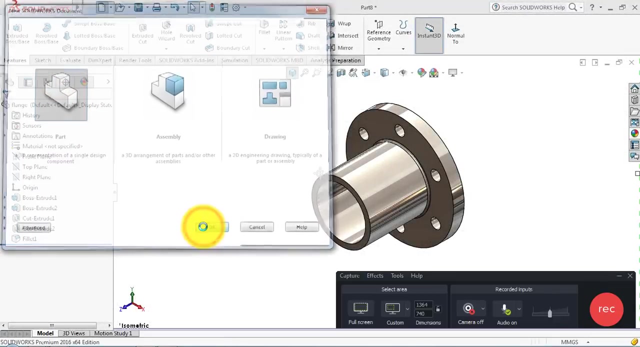 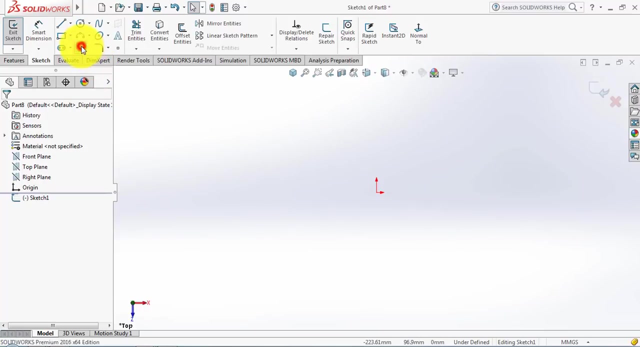 and we will name it as a flange coupling and give the name of the part as flange. ok, go to the new part. ok, now we'll go to the sketch and select here the top line. now, here we will draw hexagon using the polygon features like this and select this side and make it here. 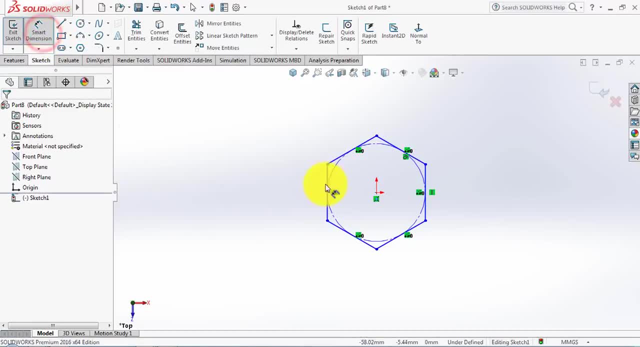 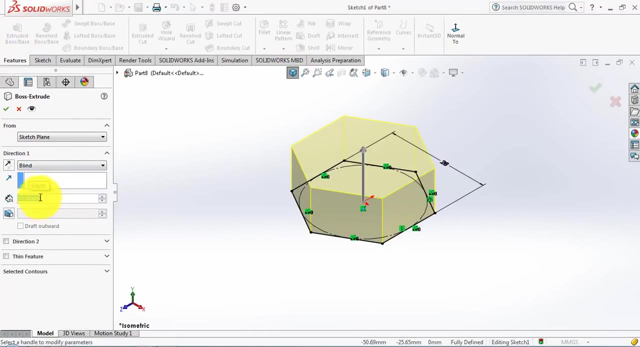 vertical. ok, now we will give it a smart dimension and give the distance between the opposite sides as 28 mm. now we'll go to the features and select its album and strict item and we will add snug of brightness to this tapabar as well- here the x-rayed boss feature and give the depth h12mm. okay, now we will go to the sketch. 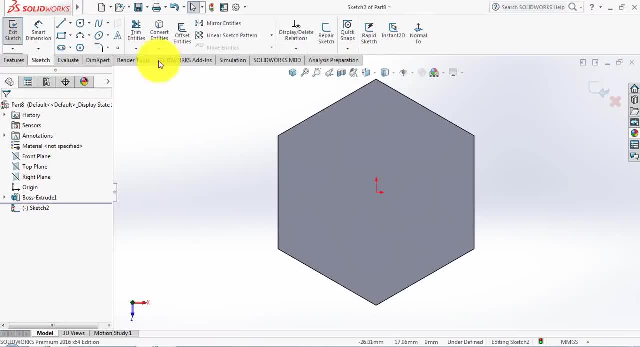 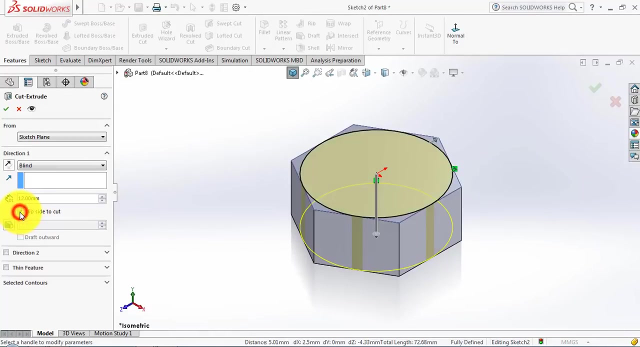 and select this face, make it normal. now here we will draw a circle like this. then select the circle, press ctrl and select this edge and make it here tangent. okay, now go to the features and select here the x-rayed cut feature. now here, select the flip side to cut. 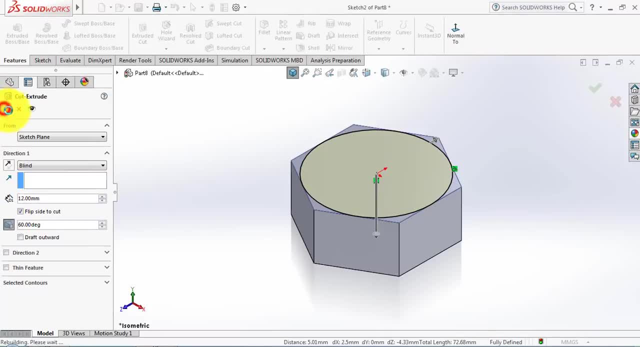 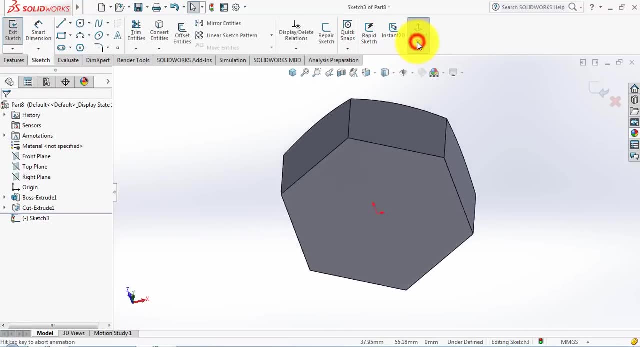 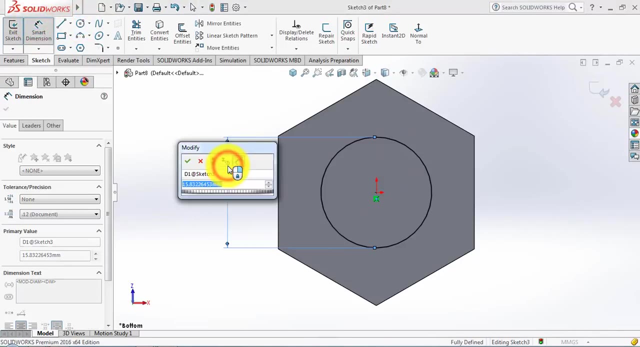 and give the draft angle as 60 degree. okay, now we will go to the sketch and select here this lower face and make it normal. now, here we will draw a circle of diameter 20 mm. now we will go to the features and select the x-rayed look section. now go to thejobs and 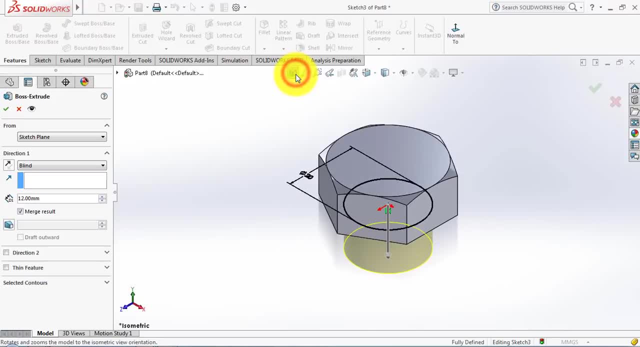 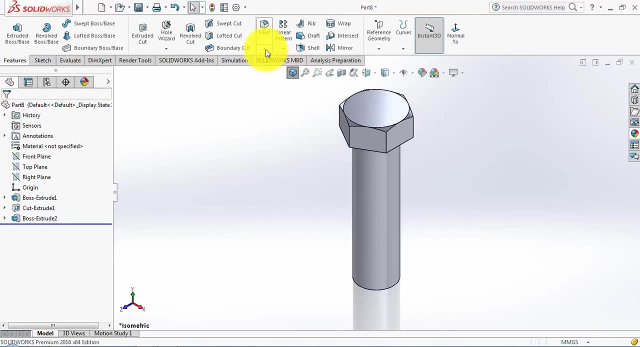 select Bell lies located here and friend chocolate used bp Tschau. you can also look at the two videos I have made earlier. give the name and color cancel, which was another good thank you for watching boost feature and give the depth as 75 mm. okay, now we'll go to the chamfer and give the chamfer. 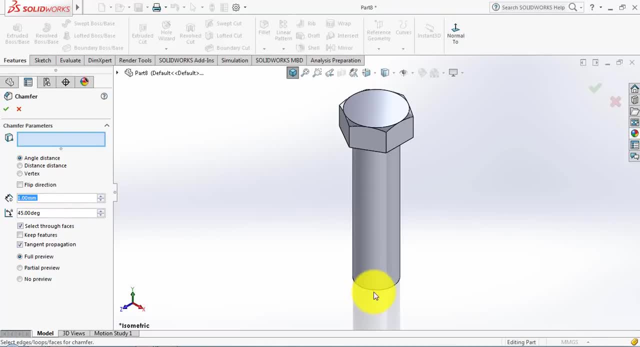 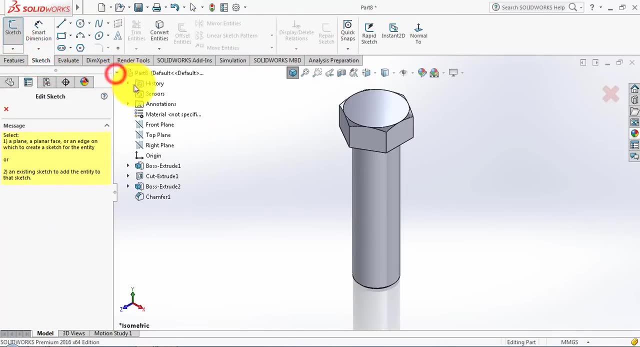 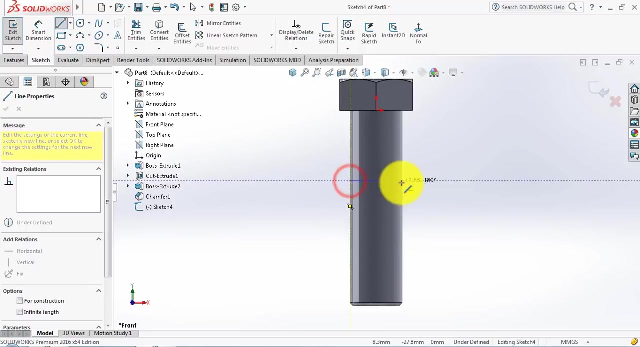 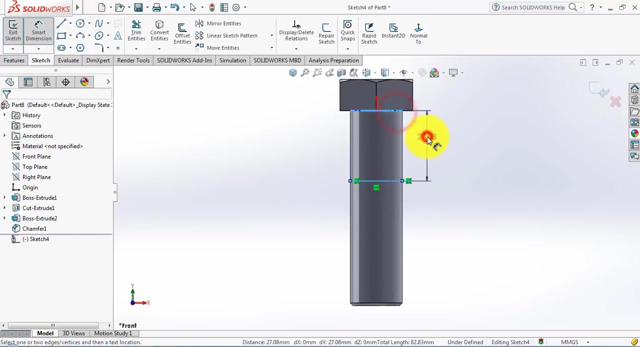 distance as 1 mm and then select here this edge. okay, now we'll go to the sketch and select here the front plane. make it normal. now, here we have to draw an horizontal line like this. now we'll go to the smart dimension and give the distance between the line and this edge as 40 mm. 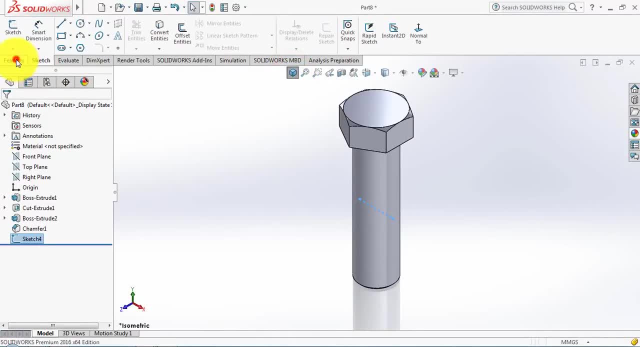 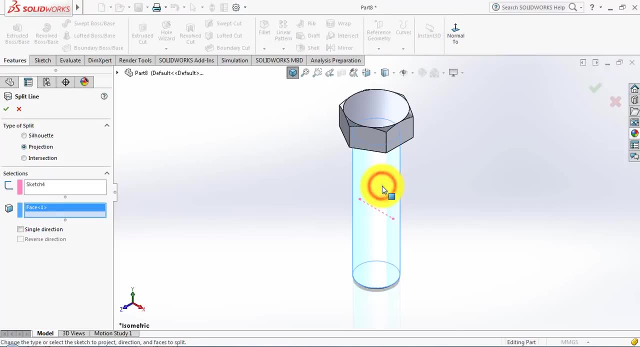 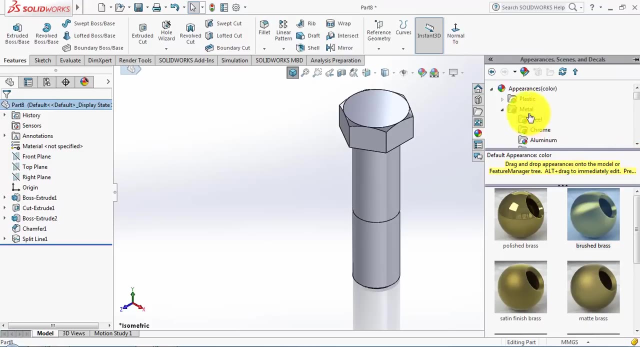 now we'll exit the sketch. then we'll go to the features and, in the curves, select here the split line and then select here the cylindrical face. okay, now select the part, go to the appearance and in the appearance, go to the metal and select here the brass. 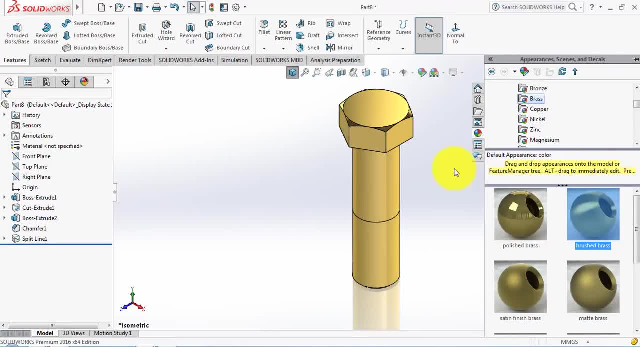 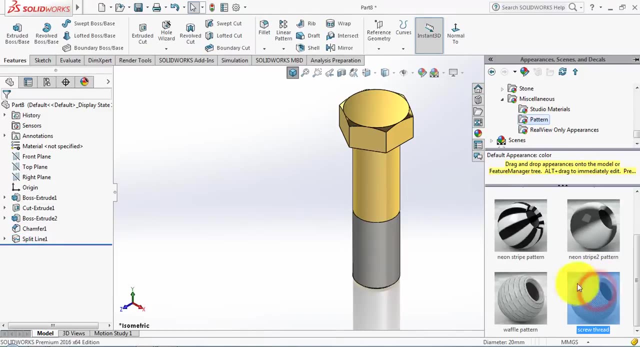 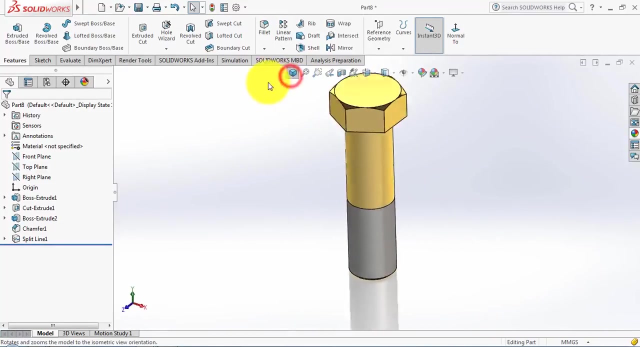 and give it the brush brush. now select this face, go to the appearance, and here we have to go for the miscellaneous and in the miscellaneous, select here the pattern and give it here the screw thread. so here you can see that the cosmetic threads are applied. and now we'll save it. so we'll go. 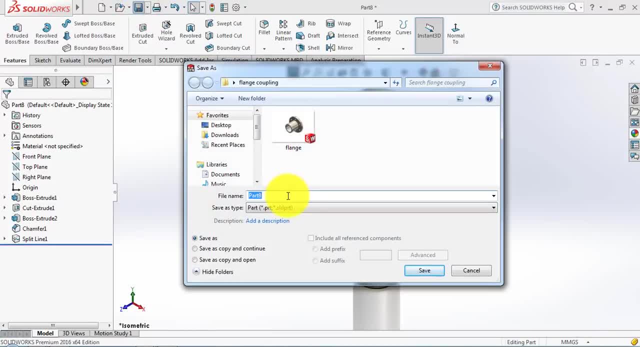 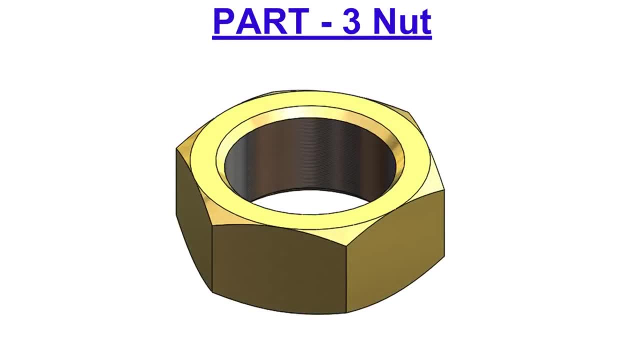 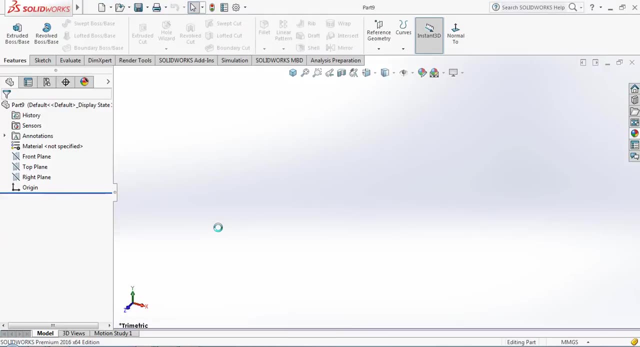 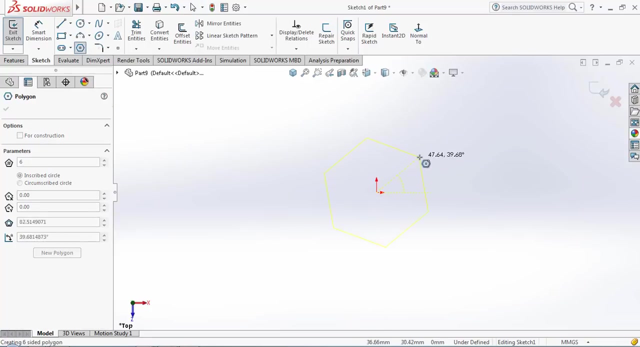 to the service and give the name of the part as bold. okay, go to the new part. okay, now we'll go to the sketch and select here the top plane. now, here we'll draw a hexagon using the polygon feature. now go to the smart dimension and give the distance between two opposite sides as 28. 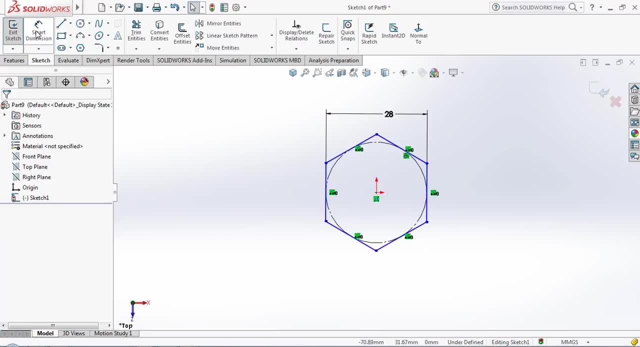 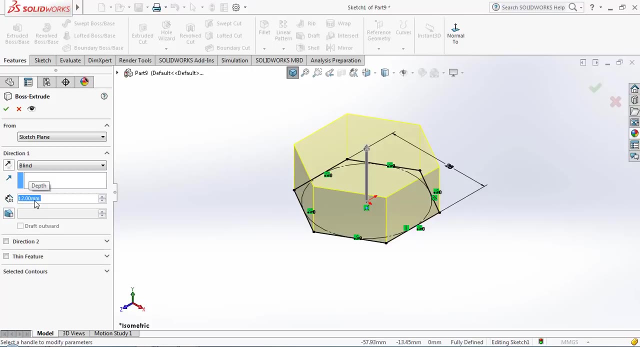 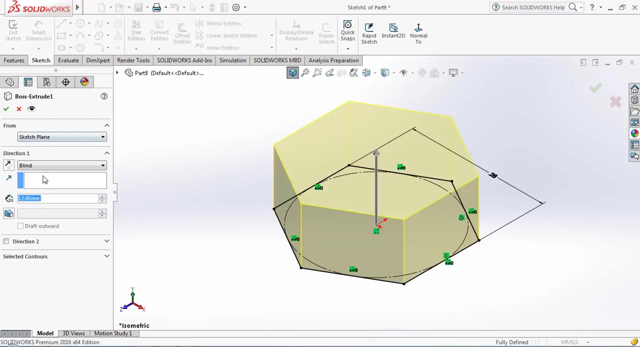 mm. now we'll exit the smart dimension now, select this line and make it here vertical. okay, now we'll go to the features and select here the extrude boss feature and give the depth as 12 mm. okay, now we'll edit the boss extrude and give it here the mid plane. 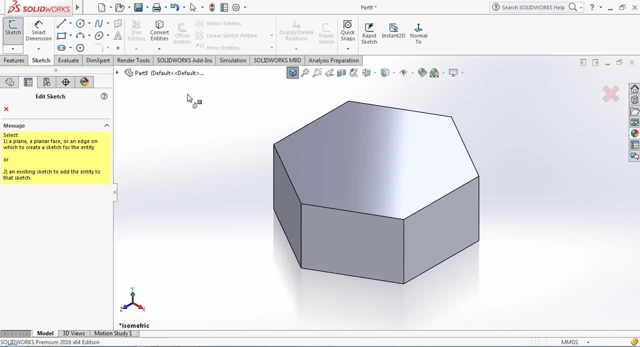 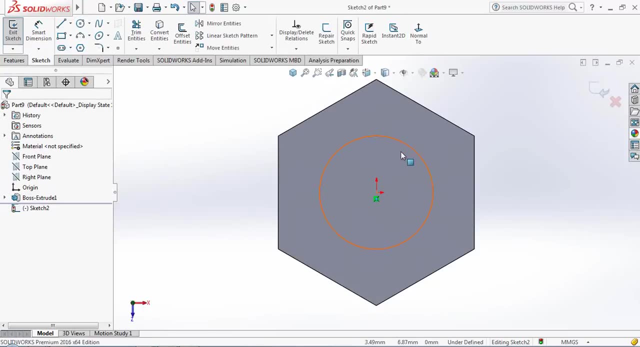 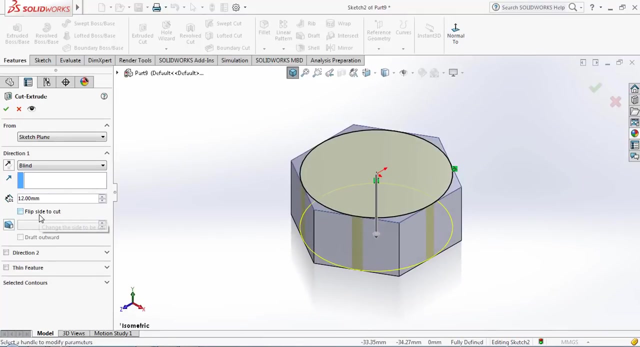 okay, now we'll go to the sketch and select this face, make it normal. now, here we will draw a circle like this. then select the circle, press ctrl and select this edge and make it here tangent. ok, now we will go to the features and select the extrude cut feature. now select here flip side to cut and give the draft angle as 60. 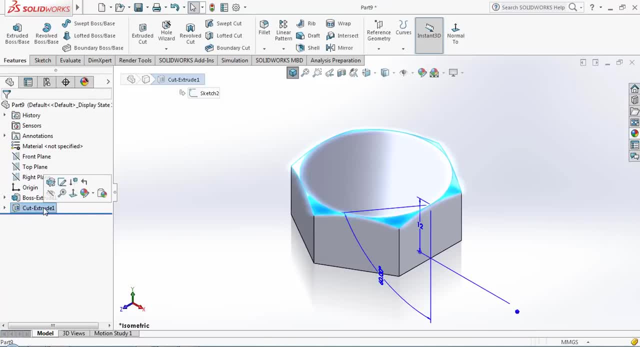 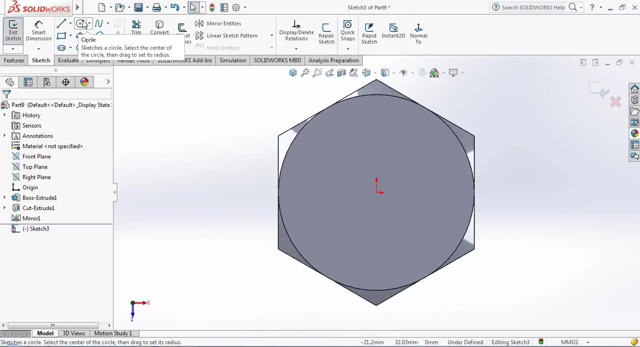 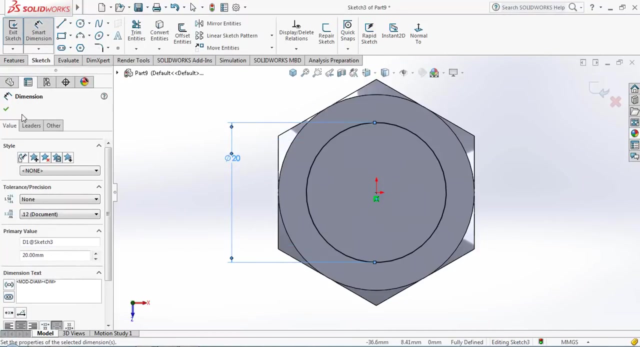 ok, now select this cut extrude and go to the mirror and select here the top plane. ok, now we will go to sketch and select the face, make it here normal. now, here we will draw a circle, last of diameter 20mm, and now we will go to the features and select the extrude. 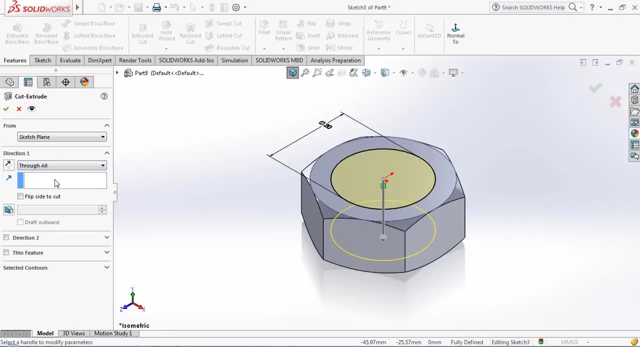 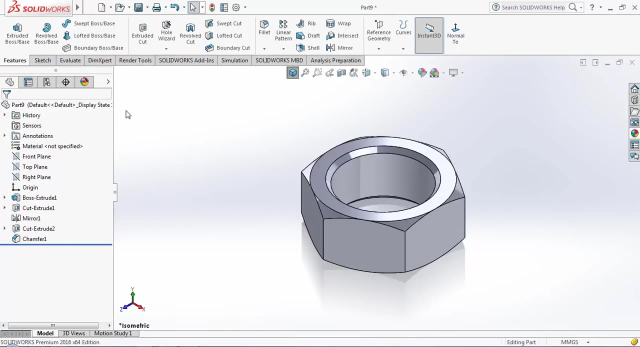 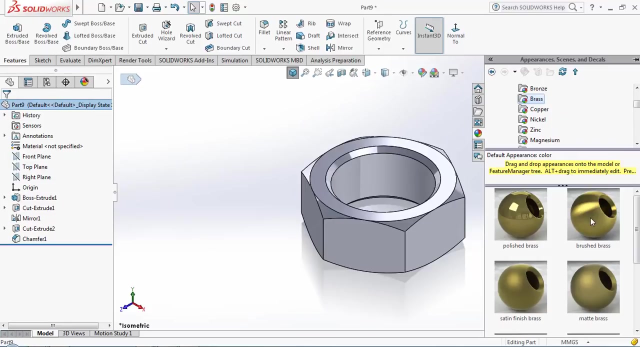 cut feature. ok, and select here through all. okay, now we'll go to the chamfer and give the chamfer distance as 1 mm and then select here this edge and this edge. okay, now select the part. go to the appearance and give it here the brush and give the brush brush. now select this surface. go to the appearance. 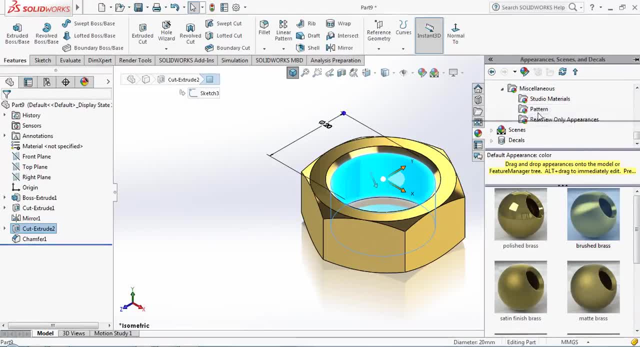 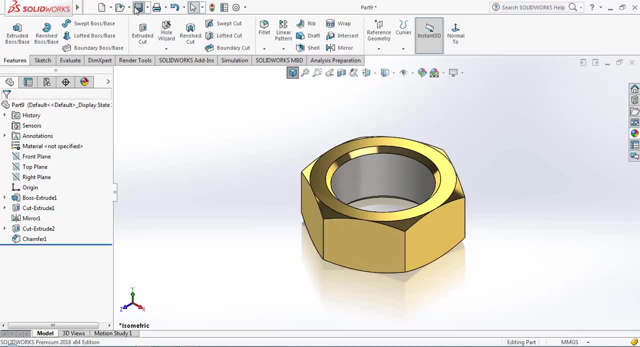 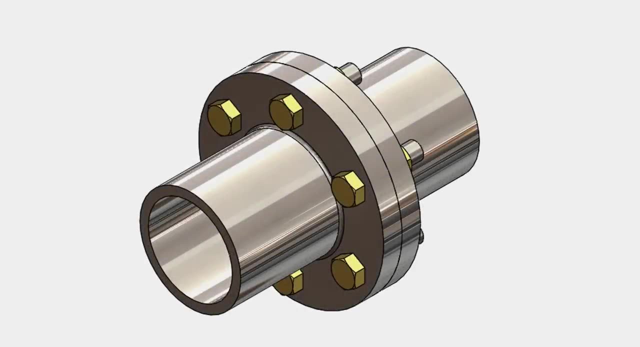 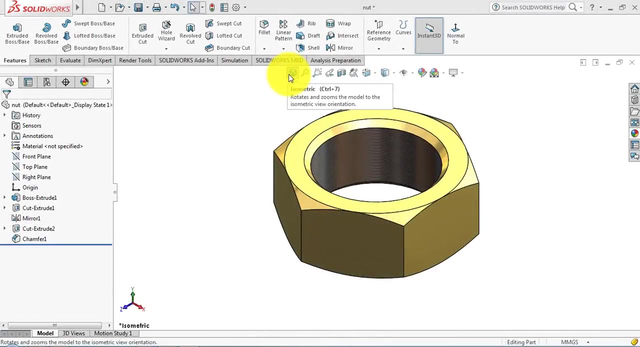 and give it here miscellaneous. go to the pattern and select here the screw thread. now we'll save it. go to the service and name the part as a knot. okay, so till now we have created all the parts, and now we are going to make assembly of all the parts, and for that we'll go to the new. 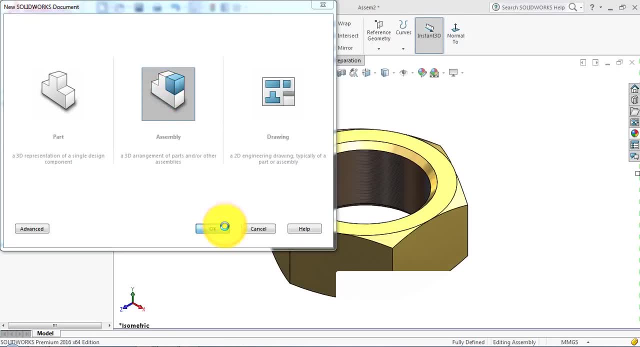 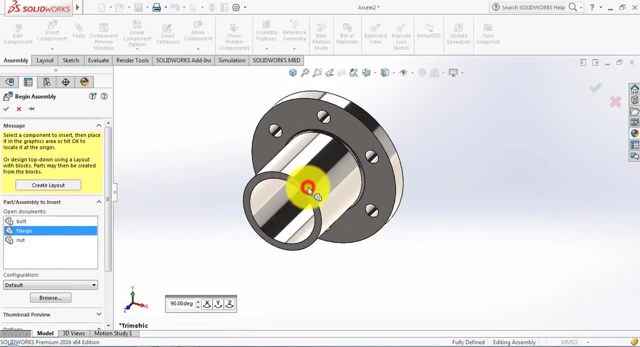 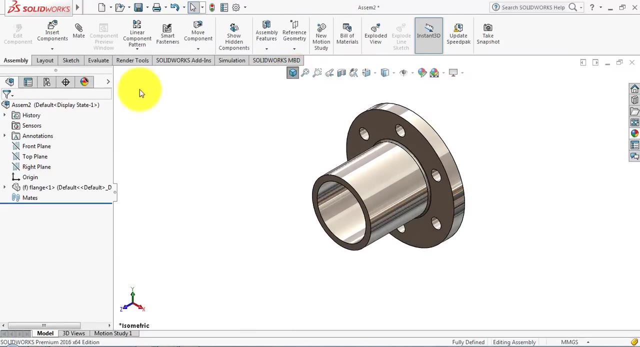 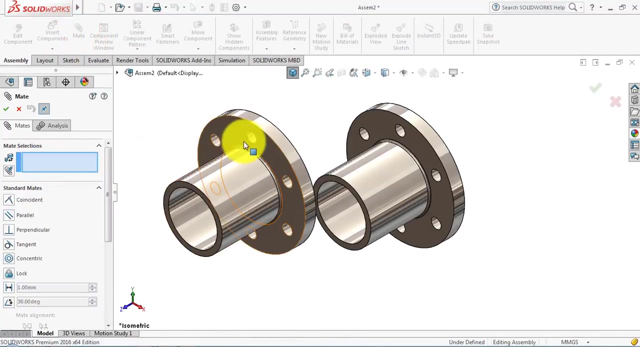 assembly and select here the assembly. okay, now first we'll import the flange like this: now we'll go to the plain white. now again we'll go to the insert component and select here the flange. now we'll go to the matte, then select here this hole and select this. 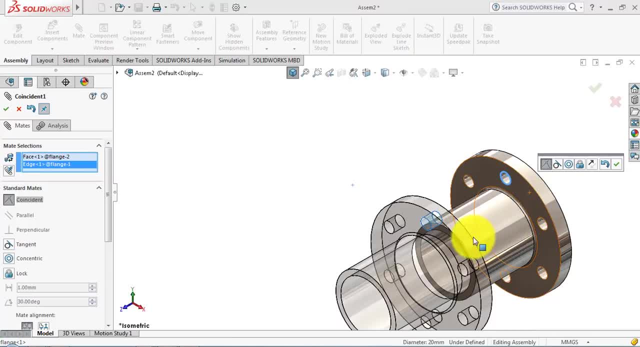 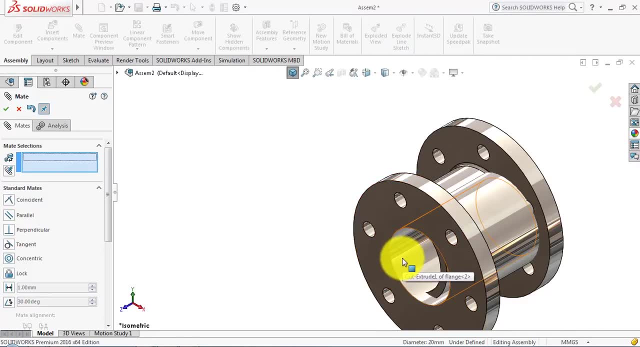 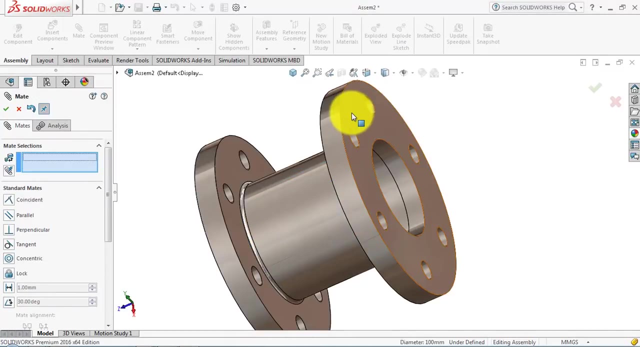 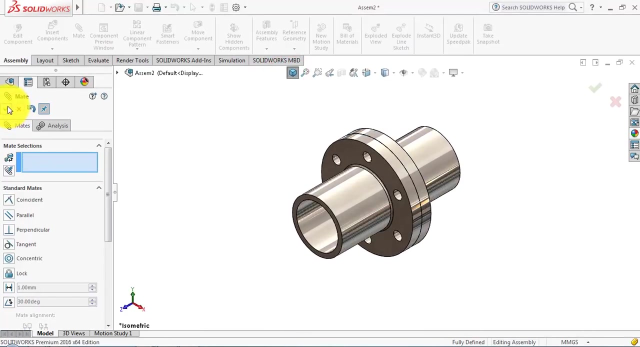 hole and here we have to give the reverse. so click on the flip matte. okay, then select here this circle and select here this face. okay, then select this face and this face. okay, now we'll close the matte. now we'll go to the new component and select here the bolt. now we'll go to the.